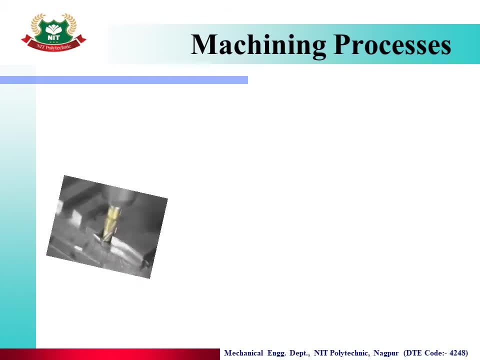 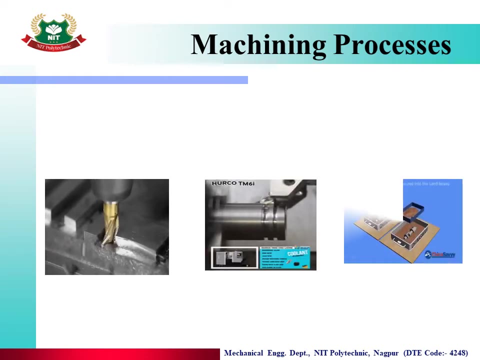 Machining process. so what is machining process? Question: that's a machining process. Take a look at this animated animation in which material is being removed. Can we call this machining process, Or can we call this machining process? or we will call it machining process. 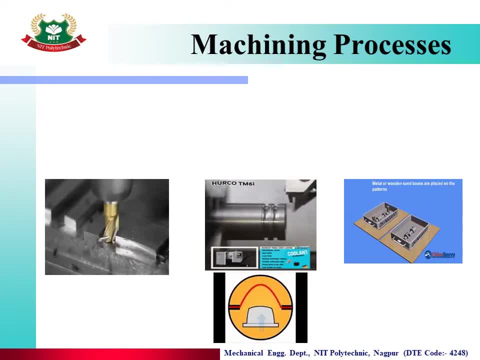 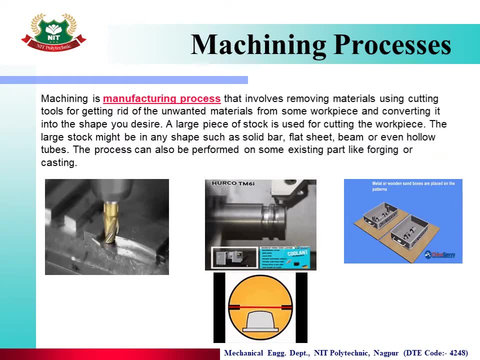 there is a might confusion. all is a machining process of different methods. so let's discuss what is machining process. machining is manufacturing process that involves removing materials, using cutting tools for getting right of unwanted materials from some work piece and converting it into the shape you desire. so machining is involved in manufacturing process. 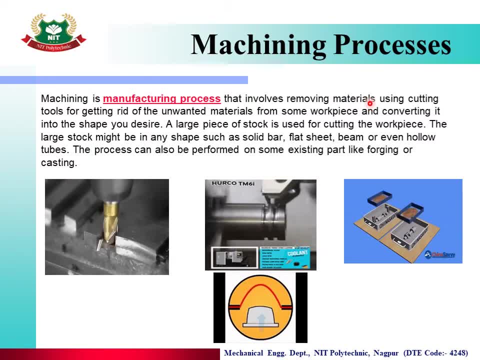 in which material is removed with the help of cutting tool. so what will happen with cutting tool? with this cutting tool or this cutting tool, material is being removed which we don't need and work piece. we will cut it. we will give desired shape, which is required. that is called as a machining process. 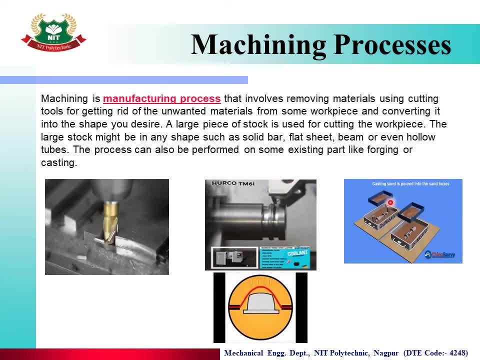 but no material is being removed in this and no material is being removed in this, so it is not machining process. let's see further. a large piece of stock is used for cutting the work piece. the large stock might be in any shape, such as solid bar, flat sheet. 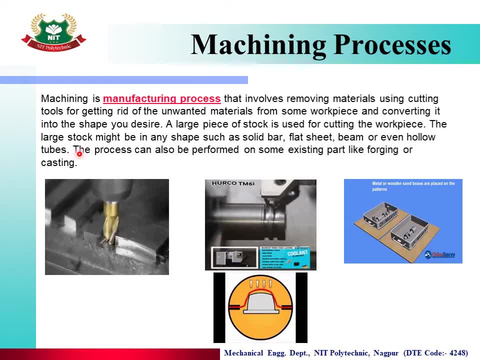 beam or even hollow tubes. the process can also be performed once some existing part, like forging or casting, so to provide desired shape material is removed with the help of tools by these processes. but to give desired shape to material we can use different methods, like this casting process. 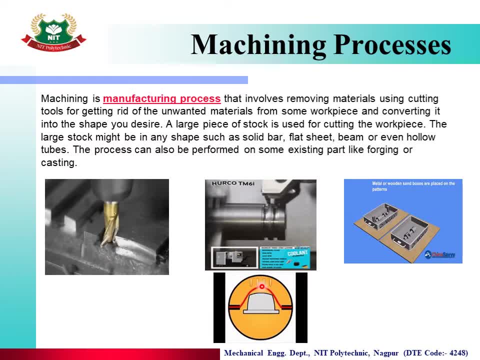 and forging process with the help of this material. material will not be removed, but desired shape will be achieved with the expansion or compression of material. so in this way we can do machining in manufacturing process. so removing material is one part, and without removing material by doing plastic deformation. 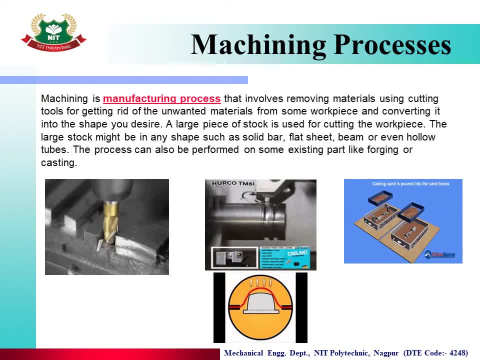 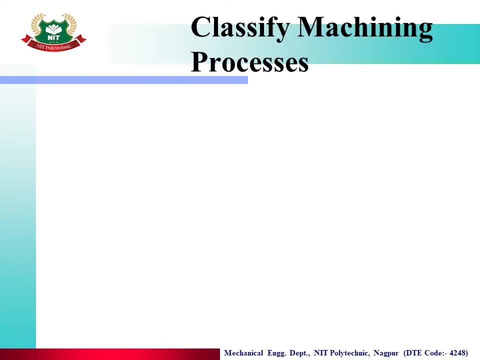 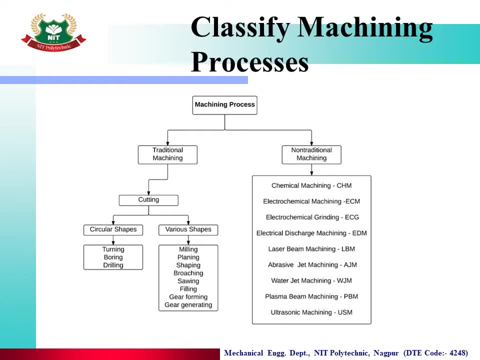 we can perform desired shape of work piece, so that is called as a machining process. let's see classification of machining process. so we have seen some types of machining process in animated form in which material can be removed in the form of chip and material is not removed. 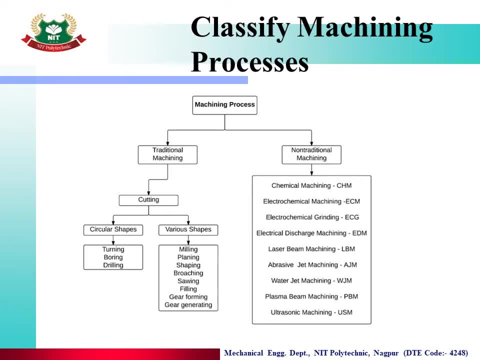 then also desired shape is achieved. similarly, machining process can be performed. we will see classification of machining process. so there are two types of machining process: traditional machining and non-traditional machining. this non-traditional machining process, in which there are various types of machining process, 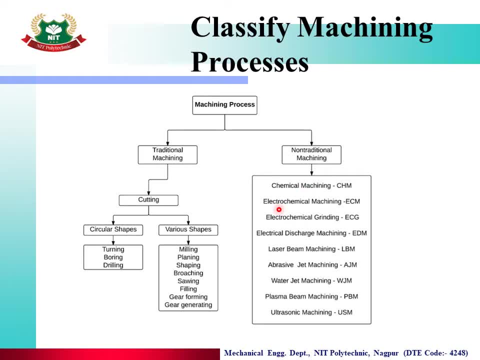 like chemical machining, electrochemical machining, electrochemical grinding, electrical discharge machining and etc. so you have to study this in advanced manufacturing process in 5th semester. so in this manufacturing process, in machining process, you have to study traditional machining. so I am not only talking about unit 1. 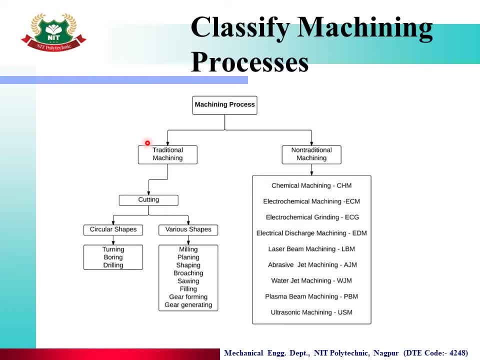 from unit 1 to 5th, all manufacturing process, machining process. that will be traditional machining process in which cutting is done. cutting is circular shape and various shape. so basically, for circular shape you use turning, boring, drilling, like shapes in which lathe machine is used. 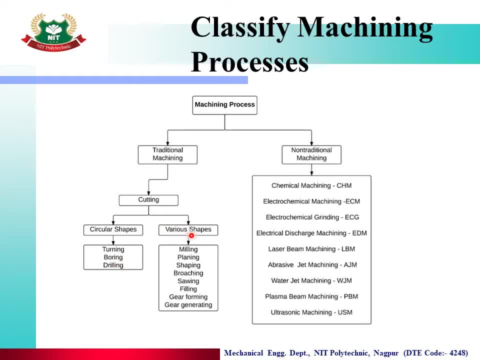 and drilling machine. and second part of cutting is various shapes. we need desired shape- rectangle, pentagon, triangle- and different cuttings in which milling, planing, shaping, broaching, saving, filling gear, boring and gear generating. so in this machining process you have to study all this in traditional machining. 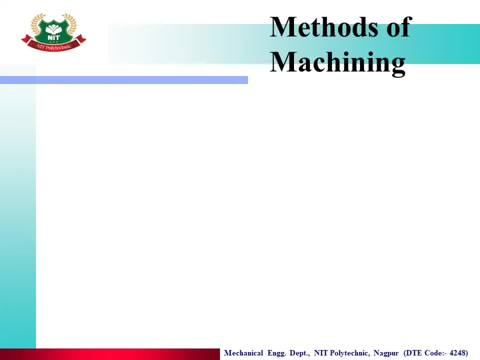 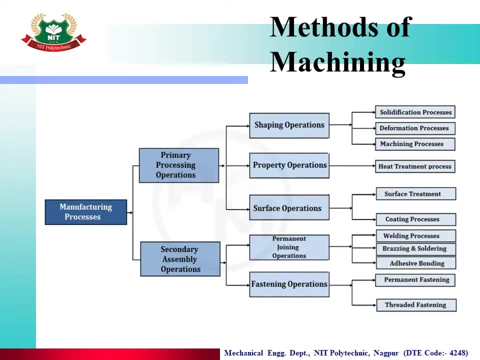 ok, so let's see next part of this, second part: methods of machining. you can call it types or you can call it classification. so in manufacturing process there are two parts: primary processing operation and secondary assembly operation. so primary processing operation is shaping operation, property operation and surface operation. 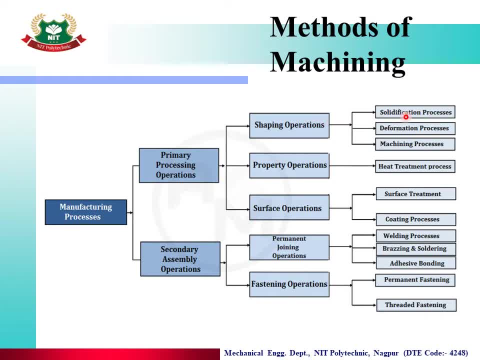 so in shaping operation comes solidification process, deformation process and machining process. so you have to study these three process through different unit. so machining process, which you will study in unit 1 and in unit 2, deformation process and solidification process, this you will study in unit 3. 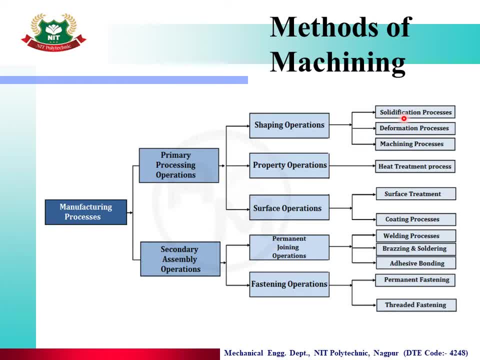 and unit 4. ok, and next we will see property operation, heat treatment process- you don't have to study here. surface operation, you don't have to study here. secondary assembly operation is your permanent joining, fastening operation. so in permanent joining process you have to study unit 5. 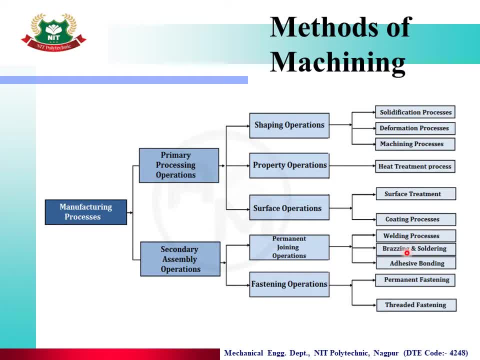 welding processes, brazing and soldering, adhesive bonding, permanent fastening, in fastening operation, permanent fastening and thread fastening. so this is our methods of machining, which is giving you introduction of manufacturing process. in short, what all it contains and in this, from unit 1 to 5: 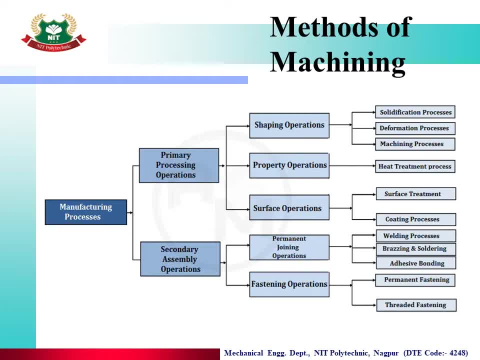 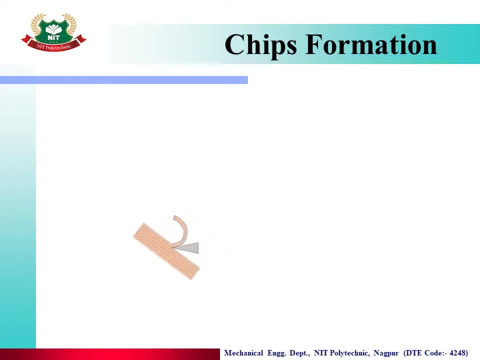 MPR syllabus is also covered. so in this, in one by one unit. next we will see chip formation. we have understood what is machining process. now we have to understand what is chip formation. what is machining process whenever we remove any material from work piece and achieve desired shape? 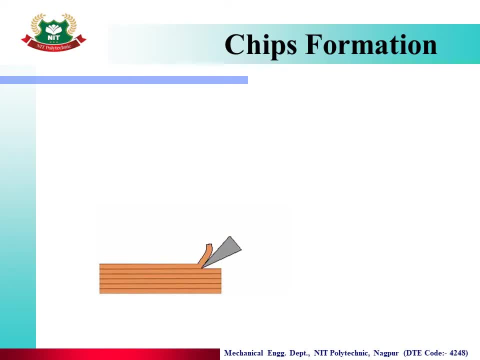 we call it machining process and operation. similarly, this machining operation and machining process, the material which will be removed, what will be in the form of chip, like this animation. you can see work piece in this animation. in work piece, tool is fitted. due to tool's movement, material is being removed. 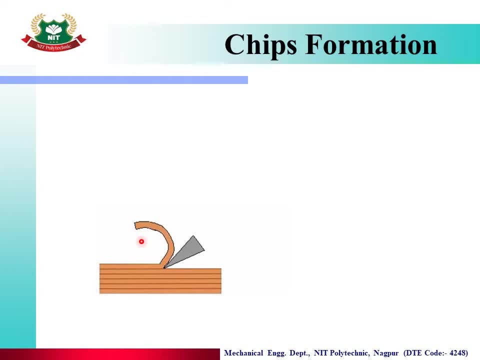 and material which is being removed in the form that is wastage. desired shape is our target, but in this material which we will remove in chip form, that is called as the chip formation. so hope you have understood chip formation and this animation is also telling you that the material which will be removed, 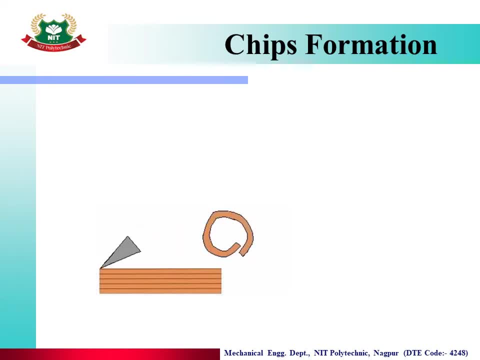 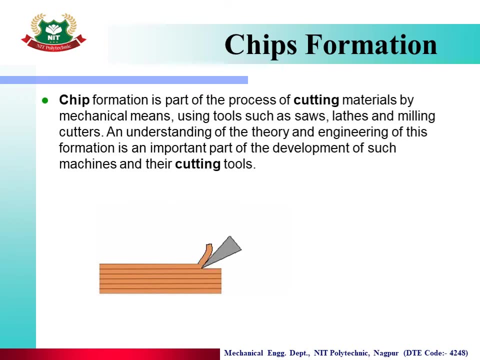 from your work, piece ok, which we will not utilize, which will not be our desired shape, that we will call as chip formation. let's see about chip formation. a chip formation is part of the process of cutting materials by mechanical means, tools such as saws, lathes and milling cutters. 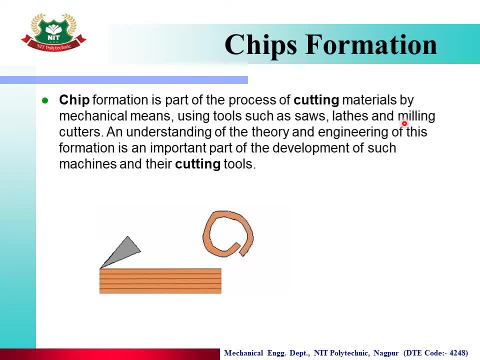 so chip formation is not of any particular machine. so, as you have seen, in first year you have worked in carpentry shop. so what you have done? you have cut wood, so what we call that. in that also wood chips are produced rounded and rounded, circular as a chip. 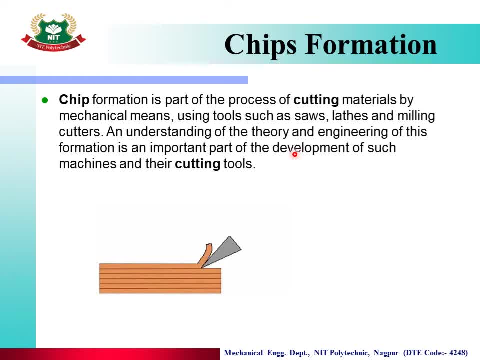 so in this different machining process, chips will be formed, and understanding of the theory and engineering of this formation is an important part of the development of such machines and their cutting tools. so the way you have to achieve desired shape, according to that cutting tool is designed and the material which is developed. 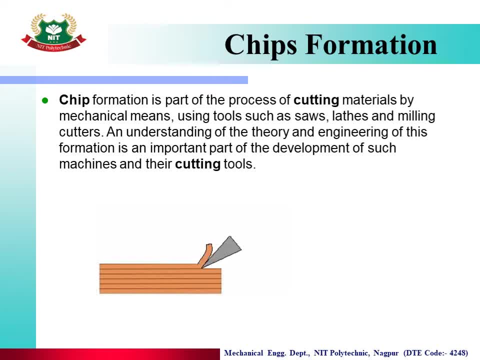 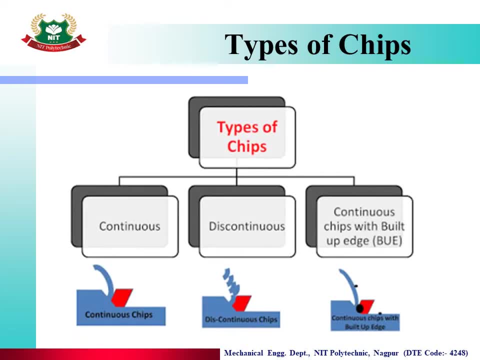 from cutting tool. we call that chip formation. let's see types of chips. so, as we have seen chips formation here, we are talking about chips which are edible, not lathes chips, particularly metal chips or wooden material chips- whatever our raw material is- which we have to convert into finished product. 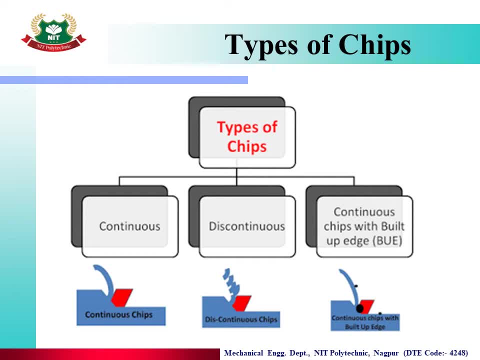 that is called as manufacturing process that convert raw material into desired shape. that chips will be formed. that is called as chip formation. and the types of chips are continuous, discontinuous and continuous chips with built of edges. below that there is a particular diagram. in continuous chips will be formed. 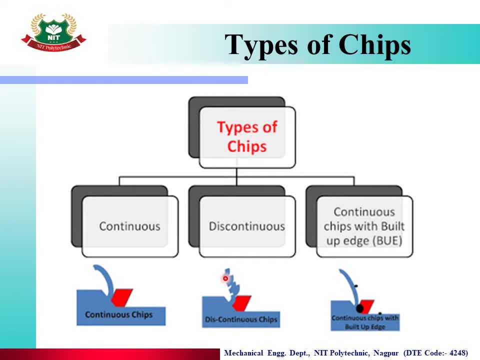 in discontinuous chips will be formed like this because we will read further, due to that, your chips will break- and continuous chips with built of edges. so in between, where edges are developed, we will call that continuous with built of edges. in notes it is continuous, discontinuous and continuous chips with built of edges. 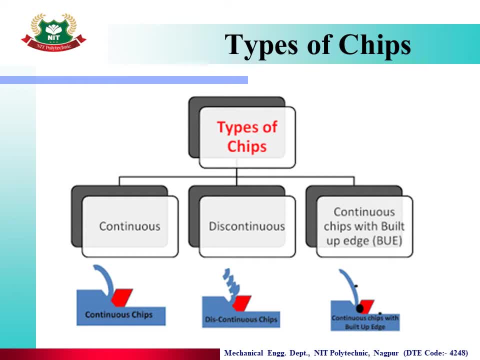 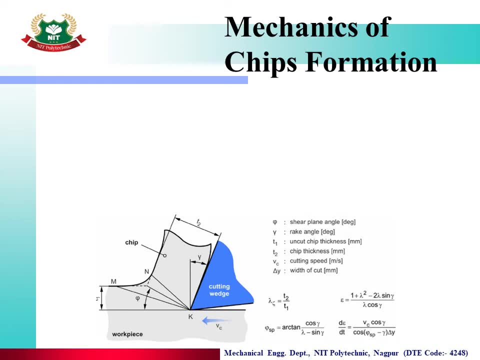 about this. you have to read a line point and you have to draw this diagram. next is mechanics and chip formation. so we have seen how chip is formed, from where chip is formed in our raw material there is chip formation and why it is happening- because we want desired shape. 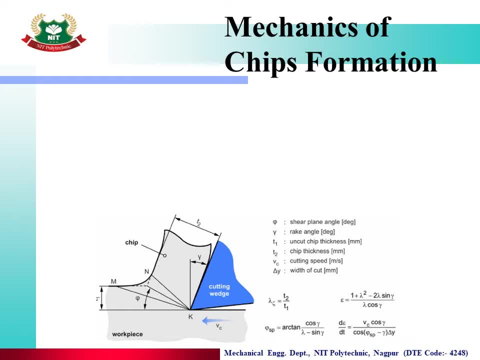 we want desired shape. so what we did? we put material in machine or hold it and, with the help of cutting tool, we removed material which we don't need. so what happened? in that material which is being removed, to achieve desired shape, chips were formed. and to form those chips, 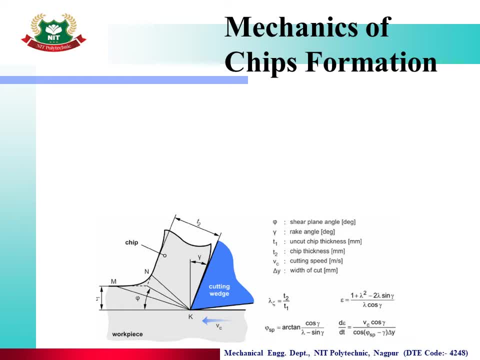 what is mechanics? why chips are forming, why it is being continuous, why it is discontinuous? there will be some logic behind it. we don't have to read derivation behind it. you note down this equation that is useful for the mechanics of chip formation. so why chip is forming? 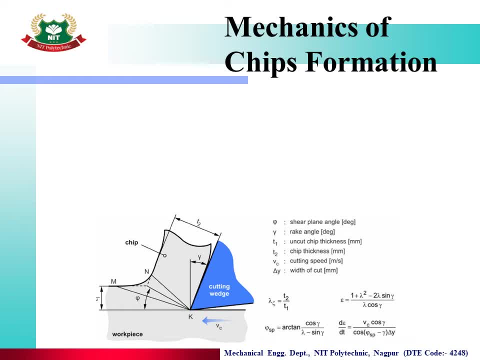 because the material of your workpiece is coming on cutting edges in that shear action is formed. ok, we have given different angles. ok, side is given shear plane angle, then gamma rack angle is given t1. is given uncut chip thickness, chip thickness, t2. this is in cutting speed. 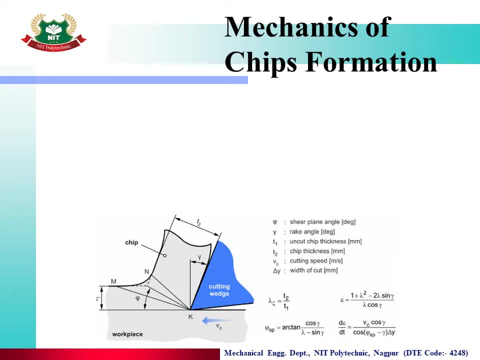 and this is the width of cut. so the width of cut and the shear plane and the rack angle depends on how your chip is developed and the formula is given here. you have to learn it because we don't have derivation in syllabus. if you read derivation, 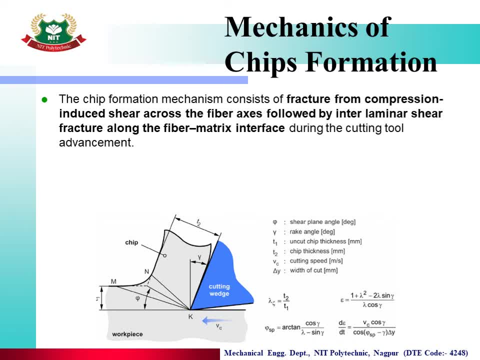 it will be complicated. for your understanding, let's see what is the mechanism for chip. the chip formation mechanism consists of fracture from compression induced shear across the fiber axis, followed by inter laminar shear fracture along the fiber matrix interface during the cutting tool. advancement when cutting tool. 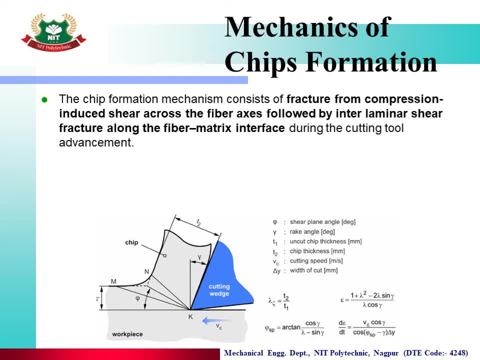 goes inside the workpiece and removes the material according to the depth of cut and width of cut. then we will see the shear of both. we will see the shear angle. we will see the shear ratio. ok, here, gamma side is given equal to t2 by t1. 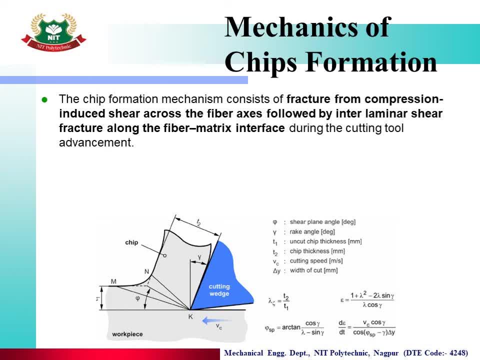 that is the difference of t2 and t1. this we will see shear action of cutting tool and workpiece, due to which we will get the mechanics of chip formation. regardless of the tool being used or the metal being cut, the chip forming process occurs by a mechanism. 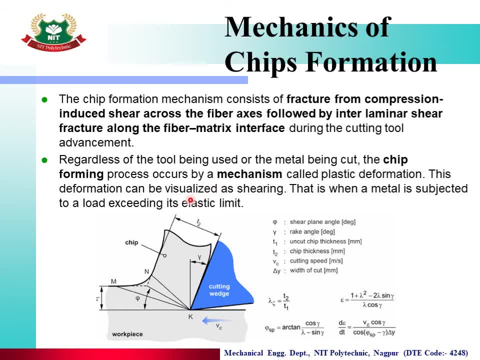 called plastic deformation. this deformation can be visualized as shearing, that is, when a metal is subjected to a load exceeding its elastic limit. when a material goes outside the elastic limit and shear, there are two pieces plastic. deformation occurs of your workpiece and chip formation is produced. 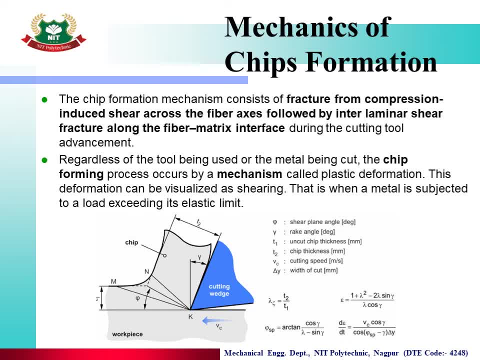 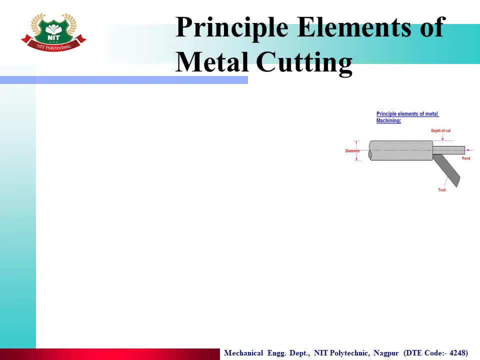 that is called mechanism of chip formation. if you have this question, then you can write these points and if you remember, then you can write this formula. so we have read the mechanism of chip formation, types of chip formation in metal. cutting and machining: what is machining? so, while doing this machining, 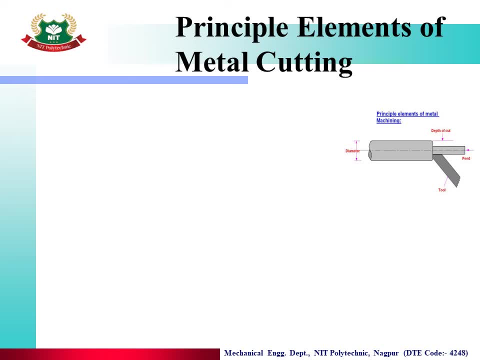 what are the principal elements you have to see? we will see here. you can see a simple diagram. on the right hand side there is a circular rod- ok- and a small bit which you have placed on the lathe machine. a lot of material is loaded on the lathe machine. 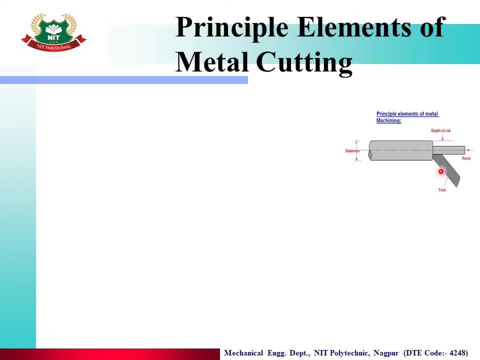 so to cut this, you will keep a tool. so when you put a tool, then what will be your diameter? diameter is the workpiece, its raw material diameter and this another diameter which you have cut. so what will be your required diameter for which you will give the feet? 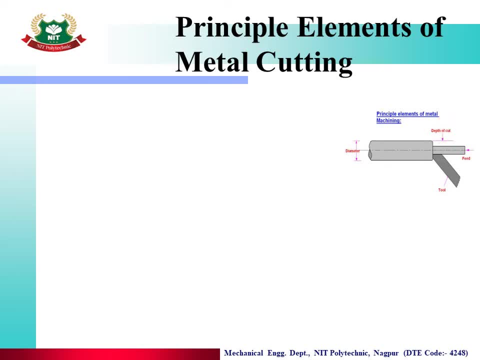 this will be your depth of dado cut will be for advanced tool movement. So let's see these things: principal elements of metal cutting. So in metal cutting, first is cutting speed. What is cutting speed? Let's see, the cutting speed can be defined as the relative surface speed between the tool and the job. So 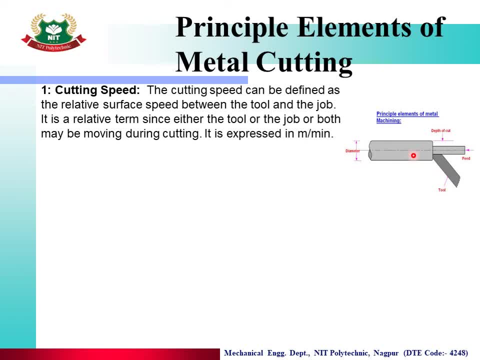 the cutting speed can be defined as the relative surface speed between the tool and the job. It is a relative term, since either the tool or the job, or both, may be moving during cutting. It is expressing the relative surface speed between the tool and the job. So in metal cutting, 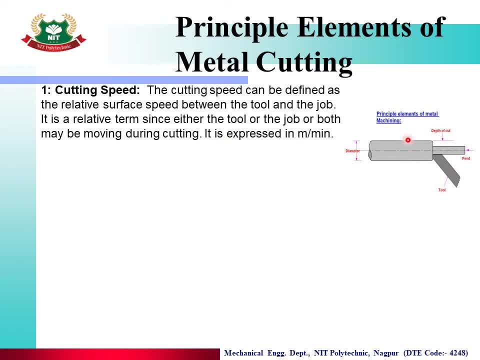 is given 5 m per minute. In this particular clip we can see that you have to calculate the rate of cut of the material in whether it is in how many meters or in how many mm, or how the material is entering into the material or how far it is going inside. So in these 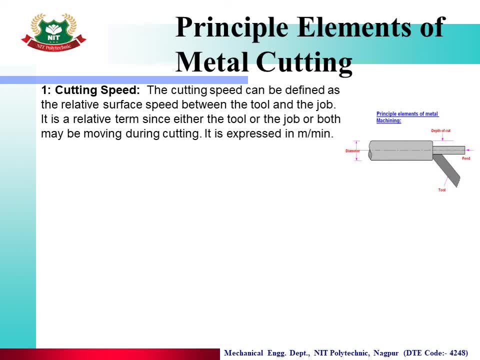 comments. you have to take into consideration the cutting speed of metal cuttings. So in this class the speed will be called is a cutting speed in the angle which rotates Next is fit. It may be defined as the relatively small cutting tool relative to the workpiece in a direction which is usually perpendicular to the cutting speed direction. 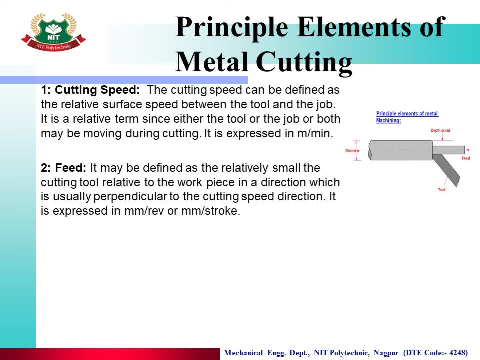 It is expressed in mm per revolution or mm per stroke. So your tool is attached to the workpiece and removing the material. So it has a feed. What is the feed? How much material will be removed in one revolution? mm per revolution. 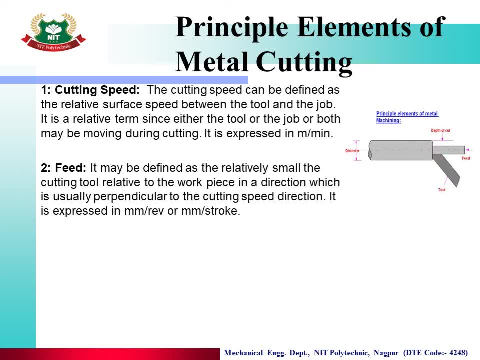 That is how much material is removed in one revolution of cutting speed from workpiece That is called as a feed. It is more complex element as compared to the cutting speed. It is expressed differently for various operations. Next is last depth of cut. 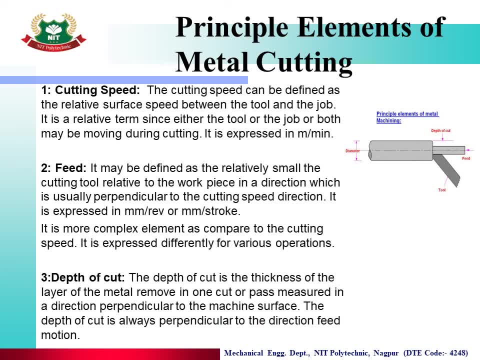 The depth of cut is the thickness of the layer of the material removed in one cut or pass, measured in a direction perpendicular to the machine surface. The depth of cut. The depth of cut is always perpendicular to the direction feed motion. So what is the depth of cut? 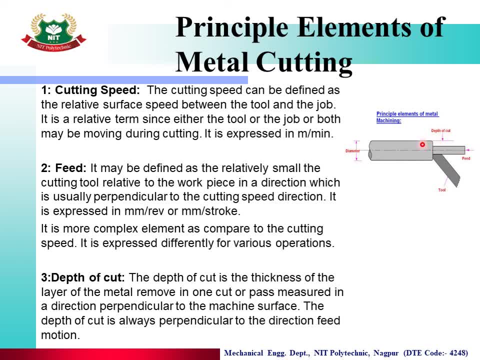 How much material is removed from this? So what is the depth of cut? If I have arranged from here to here, and I want that 1 mm is removed in one cut, then my tool set will be 0.5.. Because this object is a circular workpiece. 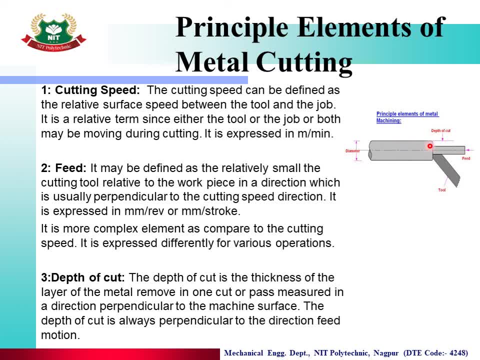 Because it is circular, it is not a workpiece, So it will be 0.5 and 0.5 or it will be removed from both sides. So my depth of cut will be 1 mm. Because 1 mm will be removed, the depth of cut will be 1 mm. 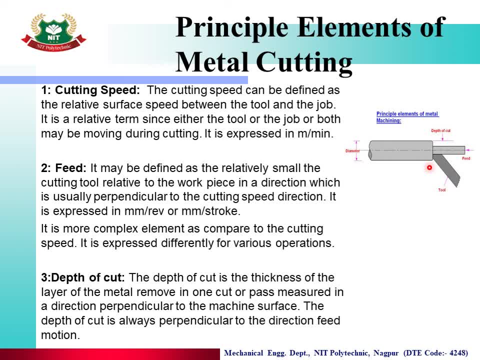 That is thickness to remove material or layer from workpiece. That is, in one moment, how much material will be removed in the form of thickness. That is called as a depth of cut. That is called as a depth of cut. That is called as a depth of cut. 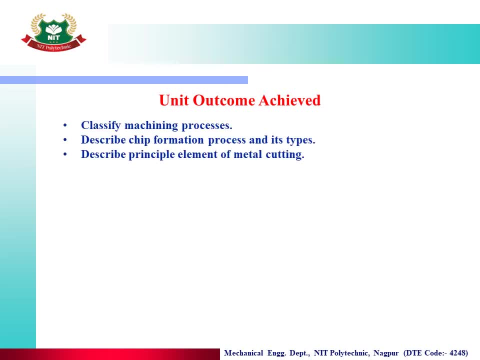 Now the time is to discuss unit outcomes achieved by this lecture as: Classified machining process. Describe chip formation process and its types. Describe principal element of metal cutting. Summary of today's lecture. we discuss Classification of machining process, chip formation process and its type, Principal element of metal cutting. 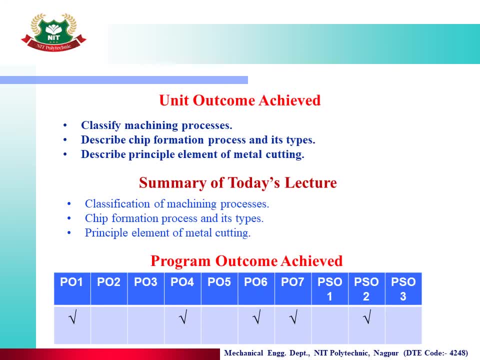 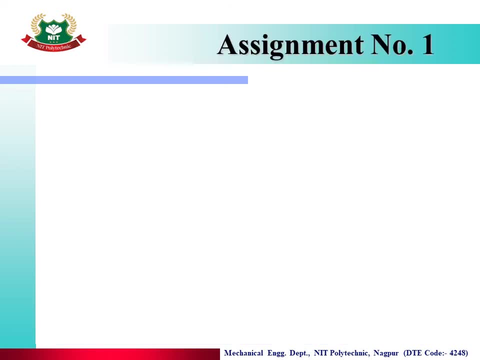 Program outcomes achieved by this lecture as PO1, PO4, PO6, PO7 and PO2 Max Assignment. Now the time is to give some assignment, and that assignment is assignment number 1.. All of you note all the questions of this assignment and solve in your class copy and